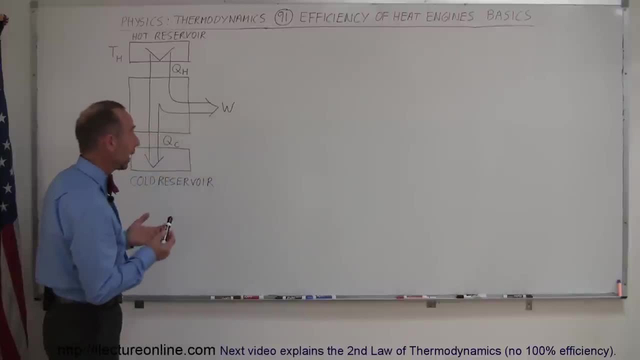 to look at is the efficiency of a heat engine. Now it turns out that in the applications around the world we use heat engines all the time. It started out with the steam engine and now, of course, internal combustion combustion engines and so forth. So a lot of applications in the world. 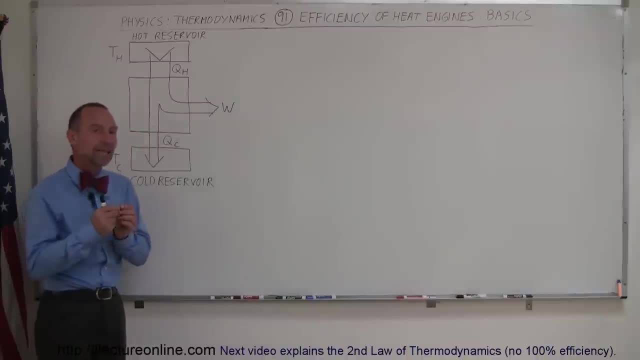 today, and the basic principle of a heat engine is that it takes advantage of the heat flow from a hot reservoir to a cold reservoir. In nature, heat typically flows from hot to cold on its own- nobody has to push it to do that- and the heat engine takes advantage of that heat flow Somehow. 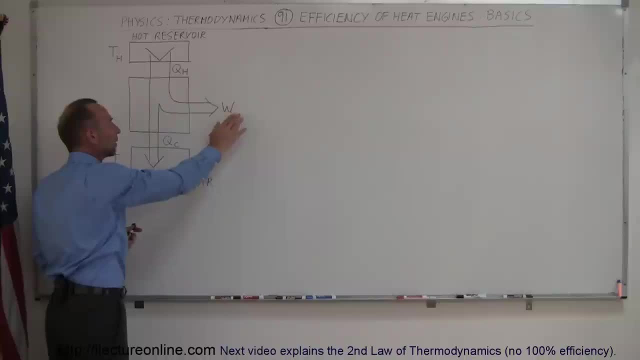 it diverts part of that heat flow and does work with it so that's that's what the w represents. Q means heat so this is the heat from the hot reservoir q sub h and the heat being expelled from that heat flow. So � turns, so this is the heat and a cycle in that cycle so 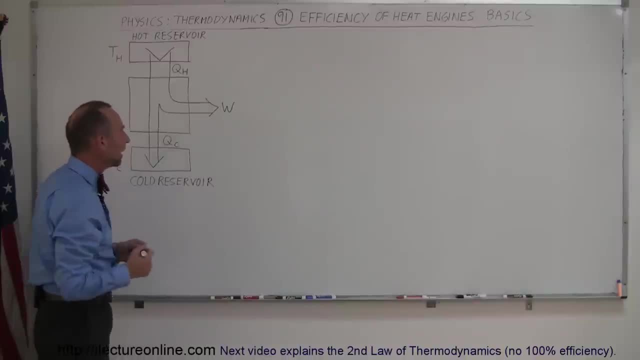 slightly more that Bea. it turns out that in December that heat takes advantage of the flow to the cold reservoir Q sub C, And the efficiency of an engine can be defined as the ratio of how much work can be done by the amount of heat that comes out of the hot reservoir. 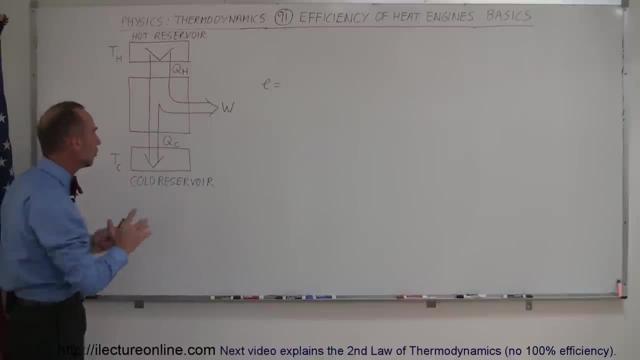 Now remember, this is simply just a graphical representation of a heat engine. Here's the engine, there's the supply of heat and there's the exhaust location, the place where we would dump the heat that is not being utilized to do work. 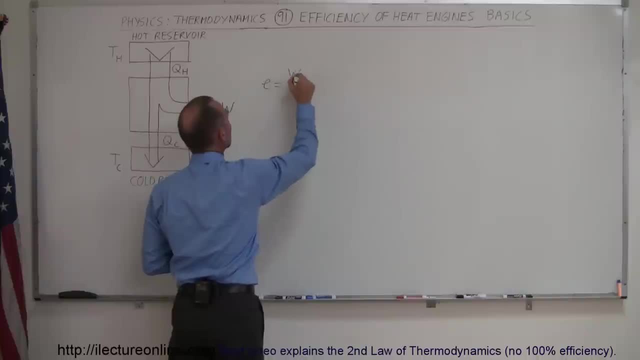 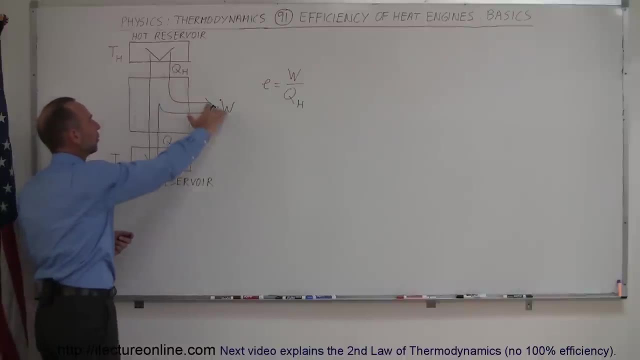 And so, by definition, the efficiency is how much work we can do divided by the amount of heat that we used on that heat transfer. Of course, the more you can divert to work, the more efficient your engine becomes. Now also, you can realize here that the amount of work that you do is simply the difference. 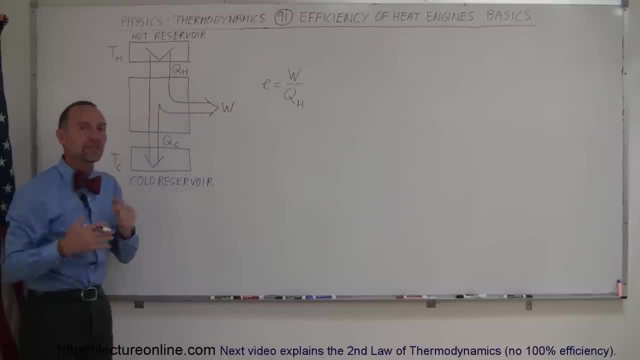 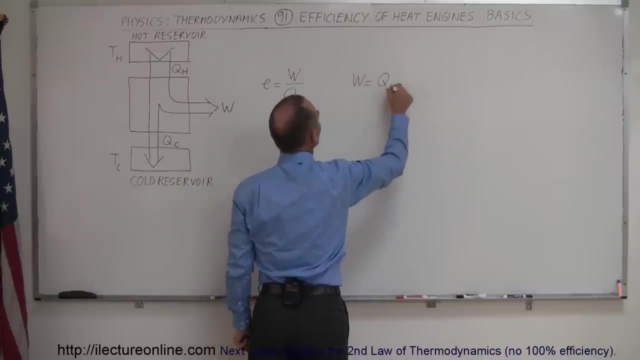 between how much heat you get from the hot reservoir and how much heat is expelled and not used to do work. So if we then use the equation that the work done is equal to Q hot minus C sub C, This Q cold, simply the difference, and we replace that in here, we can also write the: 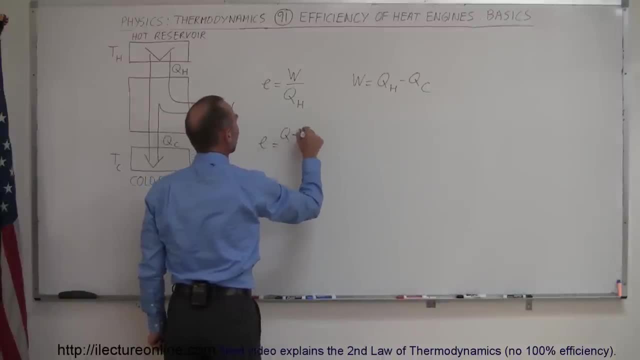 efficiency of an engine equal to the difference between Q hot and Q cold. let me write it like that: divided by the original Q hot And of course, again, if you look at it, there's two ways actually to look at it.